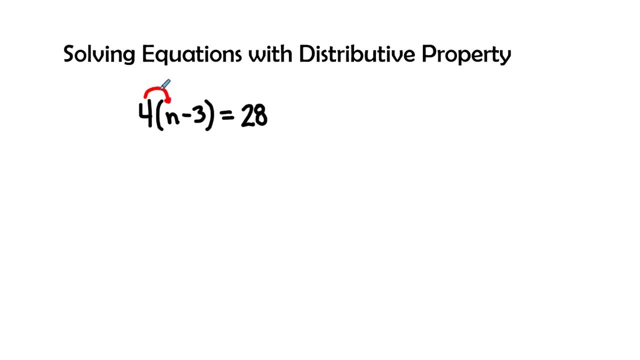 going to take this 4 and distribute it to each term on the inside of the parentheses. So here we go with our first step. 4 times n will give us 4n, 4 times a negative 3.. We always want to take the sign before the term. so 4 times a negative 3 is a negative 12.. Bring down our equal. 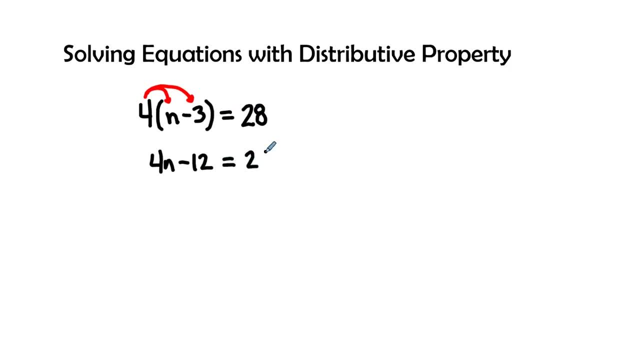 sign and the 28.. Now we have a two-step equation and we notice, with our variable we have a 4 that is attached to the variable, As well as a negative 12.. So the only way to get rid of the negative 12 and move it over to the 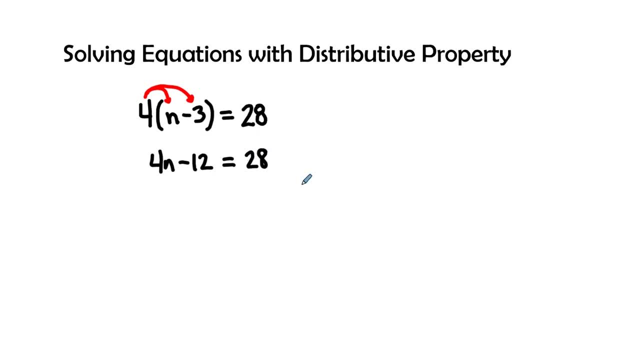 right-hand side of the equation is to add its inverse or use inverse operations. So the opposite or the inverse operation of a negative 12 is a positive 12.. And so we're going to add positive 12 to both sides of the equation. So when we go ahead, 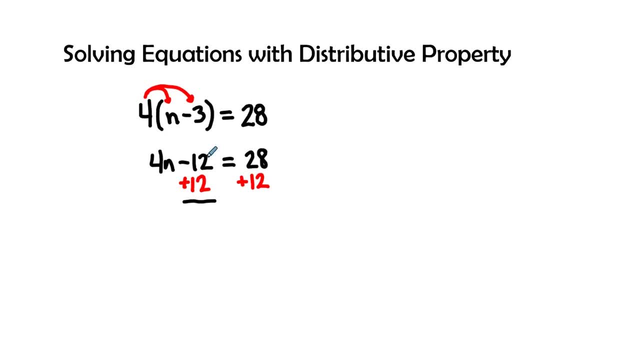 and add a negative. 12 plus 12 gives us 0.. We're going to go ahead and bring the 4n down, Bring our equal sign, And then 28 plus 12 gives us 40.. One little hint when you are solving an equation: 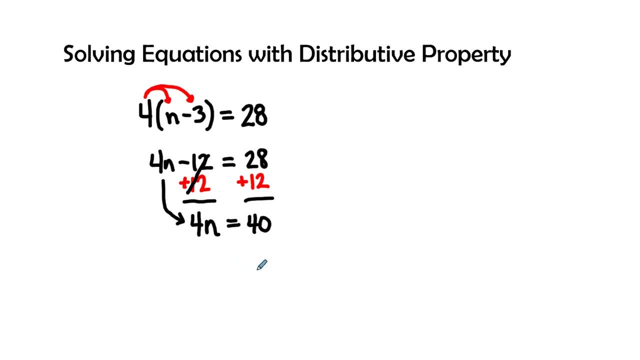 try to keep your equal signs in line with each other. It helps you be better organized and less confused. So the 4n is isolated and it's not by itself. The 4 is attached to the n. How is it attached? Well? 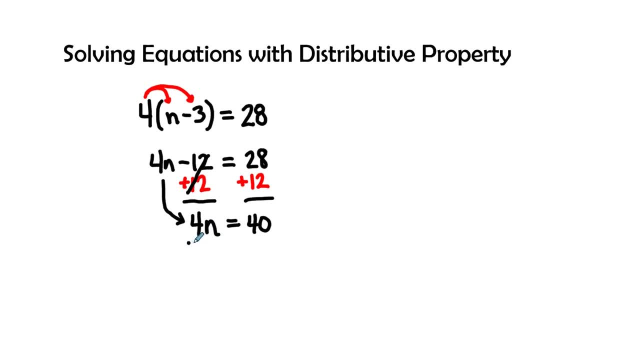 if you said multiplication, you are right. So the inverse of multiplication is division. So we're going to divide both sides by 4.. Now, 4 divided by 4 gives us 1.. So we have 1n left. We'll bring. 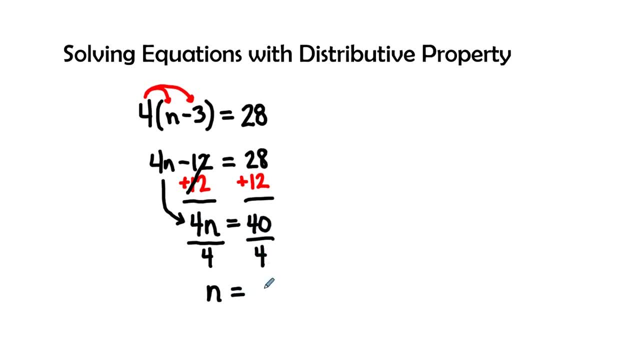 down our equal sign, And 40 divided by 4 is 10.. Therefore, the answer to this, or the solution, is n equals 10.. Now let's go ahead and check our work. It's always good to check your work when you are solving, so you know that you have the correct. 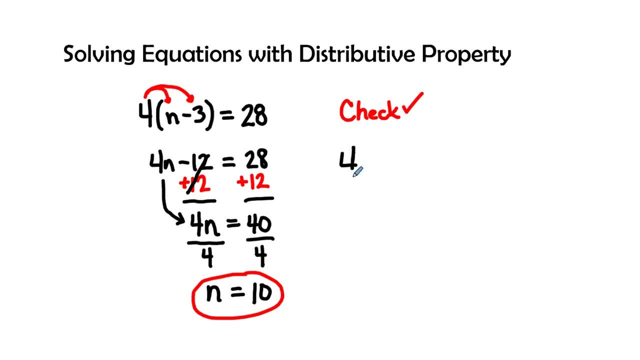 answer. So we're going to rewrite the problem And wherever we see a variable, we're going to leave a little parentheses so we can insert the number 10.. So we have 4 open parentheses. We replace the variable with parentheses, Let's plug in the 10. And we look at 10 minus 3 is 7.. So now we have 4 times 7 equals 28.. 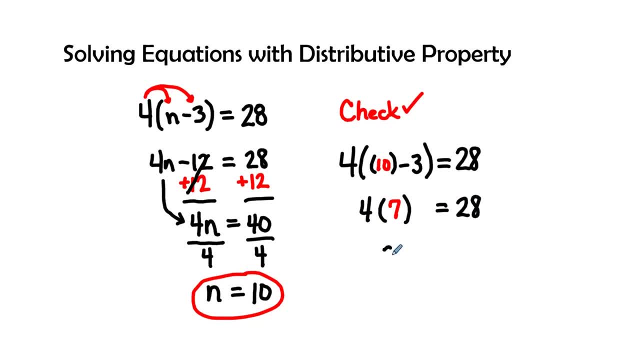 Therefore, 4 times 7 is 28.. And we are correct. When we have 28 equal to 28 or a number equal a number, we know that the equation checks The number or the solution is n equals 10.. 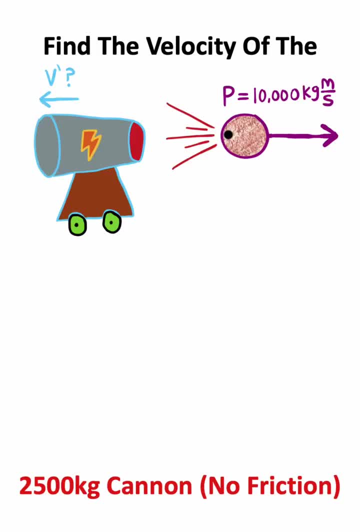 We have a cannon and the cannon launches a cannonball. We want to know what the backwards velocity of the cannon will be. Now notice how we are given the cannonball's momentum. Based on what we're given, we can use the conservation of momentum formula that says: 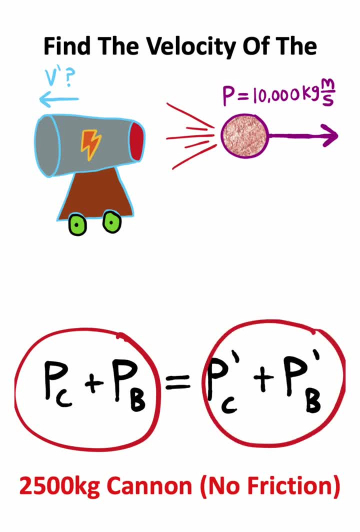 the total initial momentum is equal to the total final momentum. Now we can assume, before the cannonball gets launched, both the cannon and the ball are at rest. This means the momentum of the cannon and the momentum of the ball will both be zero initially. Now I'll take 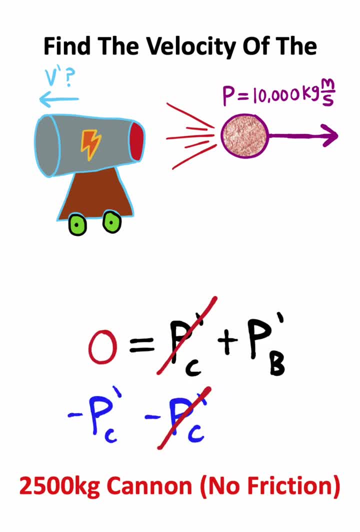 the momentum of the cannon, and I'll move it to the other side of the equation using some quick algebra. Momentum is simply the product of mass and velocity, And notice how the velocity of the cannon is what we're trying to solve for. The mass of the cannon is 2,500. 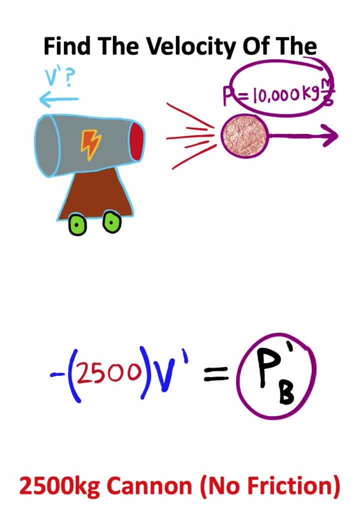 kilograms, The momentum of the ball is given to us as 10,000 kilogram meters per second. I can divide both sides of the equation by negative 2,500, giving us a velocity of negative four meters per second. So the velocity of the cannon is four meters per second in the